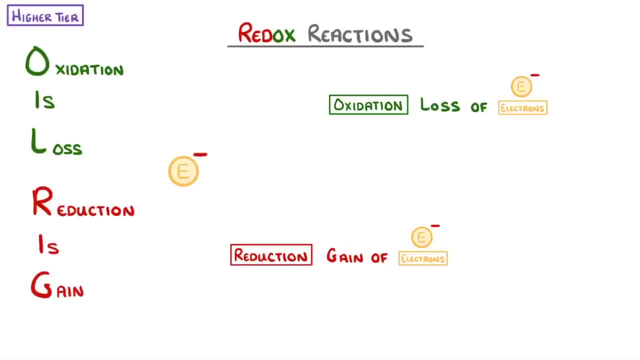 is gain, and this refers to electrons. So if we had a magnesium atom and it loses two electrons to become a 2 plus ion, then it's been oxidised, And if it gained those two electrons back, then it would have been reduced. 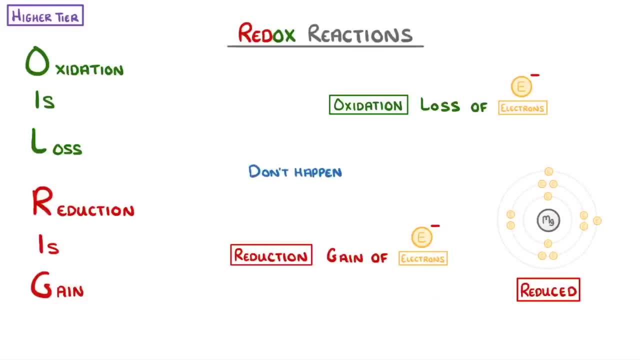 Most of the time, though, these oxidation and reduction reactions don't happen by themselves. Instead, they both take place at the same time, Because if one substance loses electrons, then another substance has to gain them. And because both happen together, we call 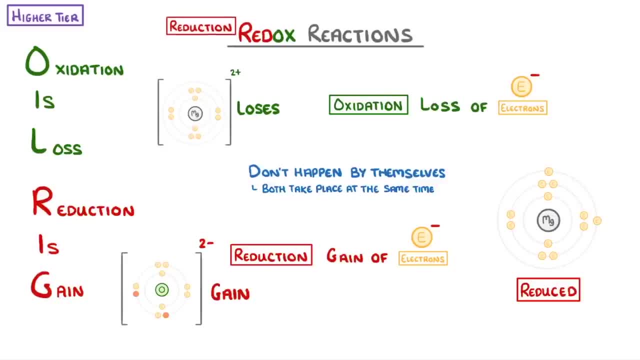 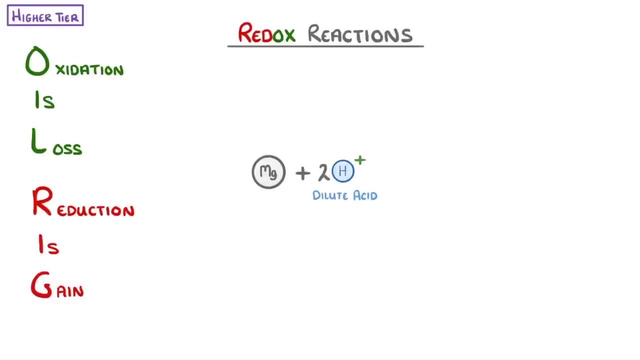 them redox reactions, which just means reduction-oxidation reactions. For example, if we react some magnesium with a dilute acid which we can represent as H+, because that's the important part of an acid, then the magnesium atoms will lose two electrons. 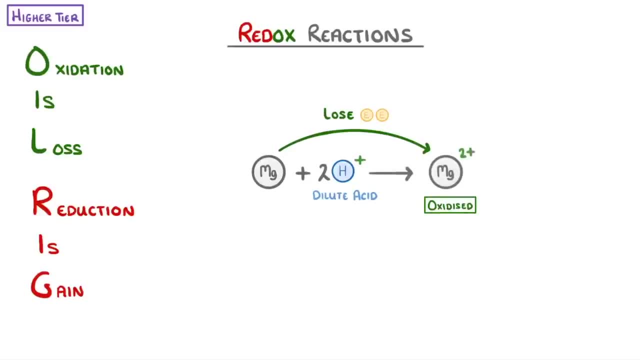 and be oxidised, forming magnesium 2 plus ions. Meanwhile, the hydrogen ions will gain those electrons and so be reduced to neutral hydrogen atoms in the form of hydrogen gas. Another place we see redox reactions is in displacement reactions which involve a more 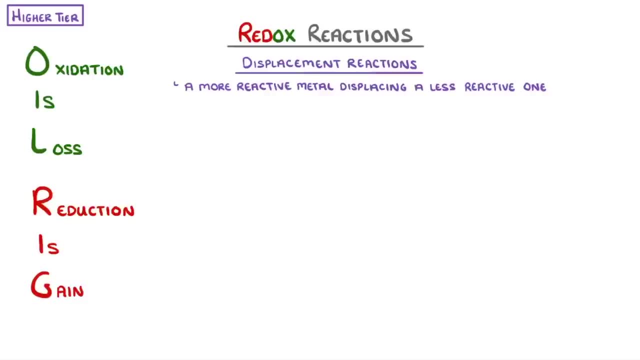 reactive metal displacing a less reactive one. For example, if we look at out reactivity series, we can see that calcium is more reactive than iron. So if we added some calcium to a solution of iron sulphate, then our reaction would take place with some calcium until it. 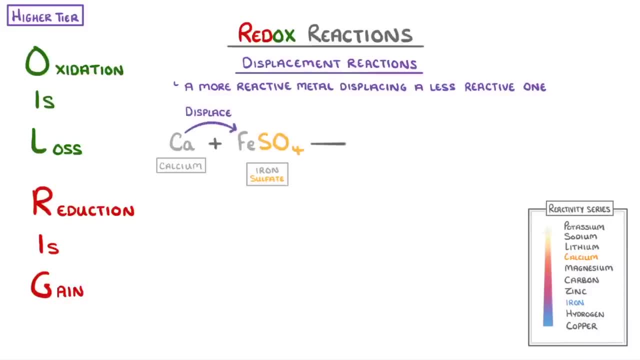 ensures the reaction is important, then the calcium would displace the iron to form calcium sulphate, while the iron would precipitate out as a solid. For reactions like this, it's sometimes useful to write them as ionic equations, in which we only show the particles that actually take place in the reaction and change in. 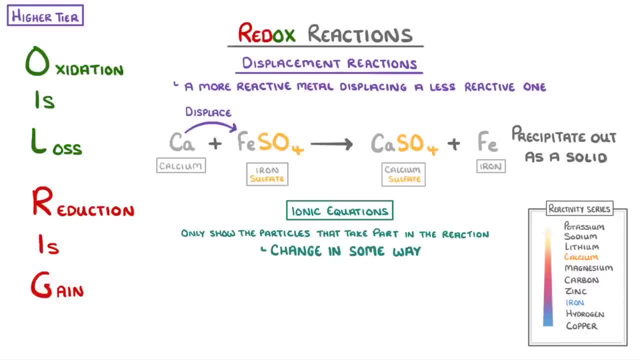 some way. For example, if we showed everything here as ions, we can see that the sulphate ions stay as SO2- ions. They don't actually change or take place in the reaction by exchanging electrons. Because of this, we call them spectator ions and get rid of them from our equation.